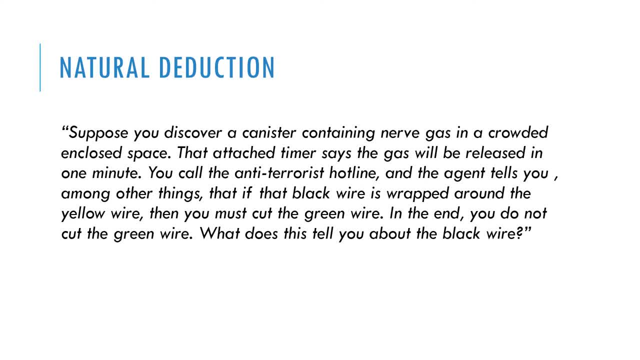 that if that black wire is wrapped around the yellow wire, then you must cut the green wire. In the end, you don't cut the green wire. The question is, what does this tell you about the black wire? It should tell you that the black wire is not wrapped around the yellow wire. 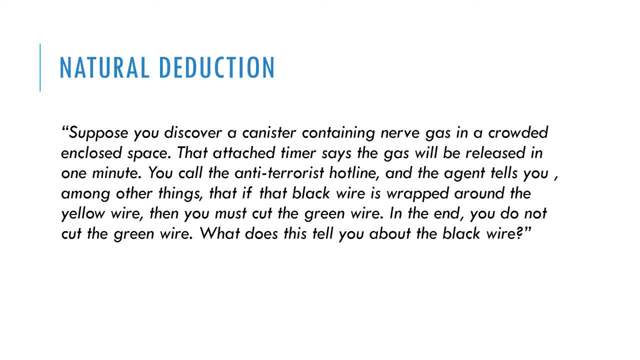 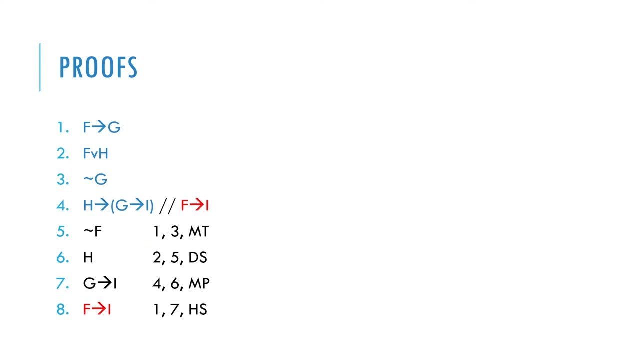 But how is it that we know that? We know that because we go through in our head a series of natural deductive steps that justifies how our reasoning leads to our conclusion. Here's an example of such a proof. Now, this is a much more complicated argument, and one that essentially does the same thing. 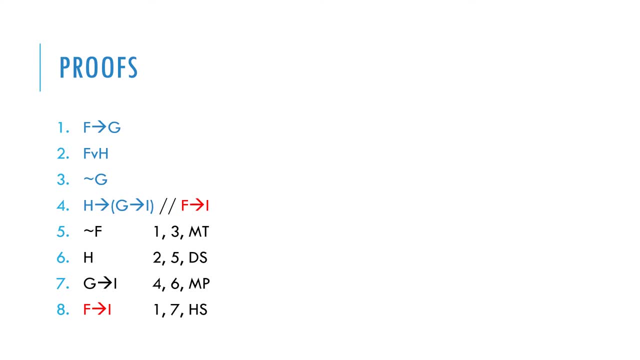 So if you look at the argument initially in lines 1 through 4, the premises are in blue, the conclusion if F, then I, in red. So we know that if F then I is true, we can see that we have a negative conclusion. that leads us to the point where we can make that case through. 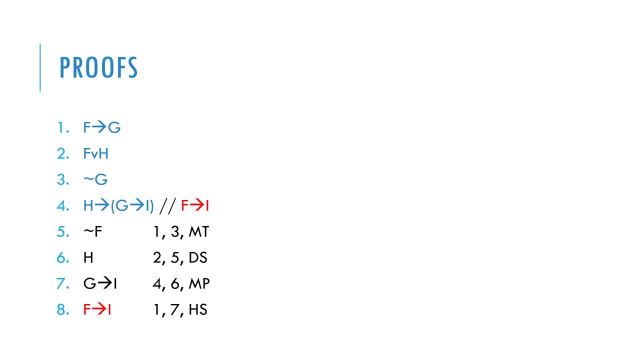 the same series of deductive steps that we solved the last problem, And here we can back that up and show how we get from each premise to new information. that leads us to the conclusion. So if we look at this argument- 1 through 4,- 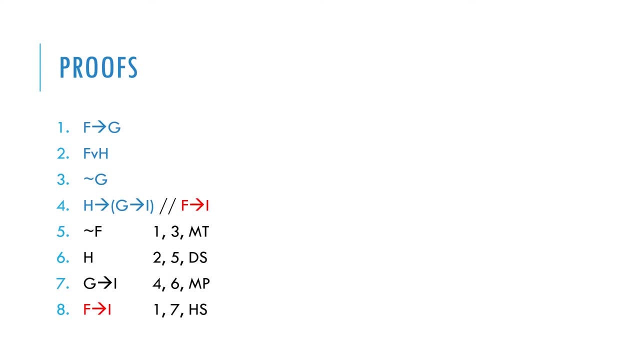 leading us to: if F then I, we can see that my justification, based on steps or based on lines one and based on lines three, i know that not f is true and i know that not f is true in line five because of a natural deductive uh inference known as modus. 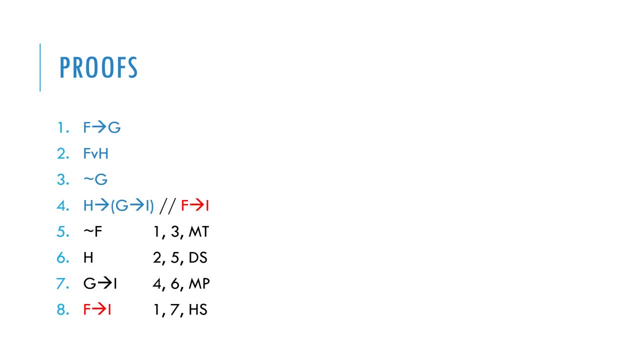 tollens, something that we're going to look at in this lecture. once i know that not f is true, then i can use line two and line five through a step called disjunctive syllogism to get line six and know that h is true using line six and line four. i know that if g, then i is true. 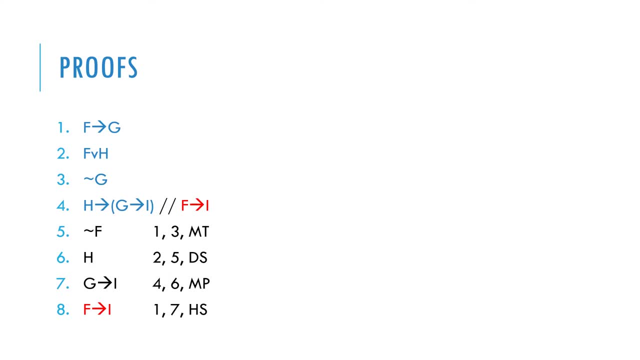 through the inferential step of modus ponens. and then lines one and seven get us to know that if f, then i, which is our conclusion, through the inferential step of hypothetical syllogism. so here i can justify all of my natural deductive steps that lead me to my 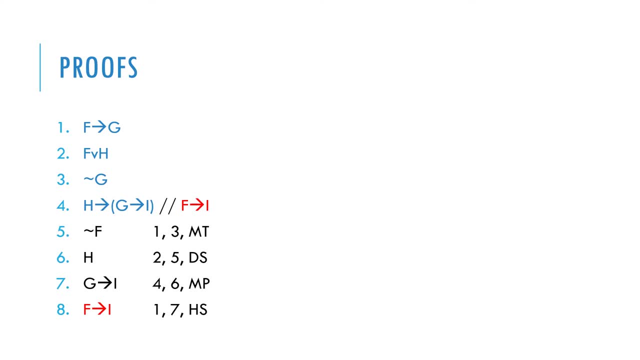 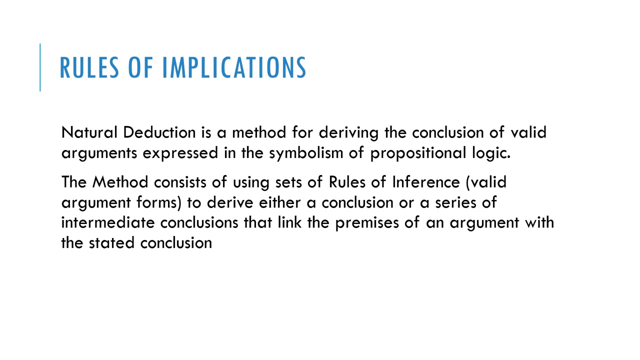 conclusion, through these justifications, of knowing how to do this type of proof, which is what we're going to be doing in the next two modules. natural deduction is thus a method for deriving a conclusion of valid arguments expressed in propositional logic. so what that means is that when i have a valid argument, i can justify. 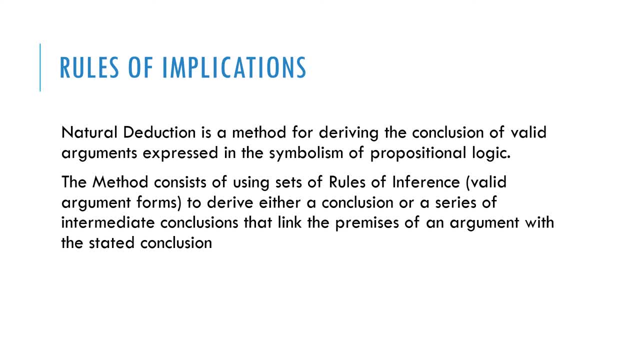 certain steps that will deduce certain other conclusions, or i can justify my conclusion based on differing steps that might be different from my natural deduction. so i can justifying separate steps. with talked if is a égal term, it deer does relate to different distances, different terms of誰. 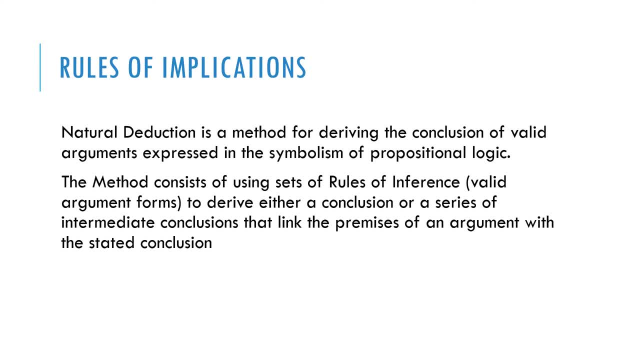 that can be explored within these proofs. so the method consists of using sets of rules. these sets of rules are rules such as modus ponens and modus tollens, and these are rules of inference- valid argument forms- so to derive either a conclusion or a series of immediate intermediate conclusions that link these. 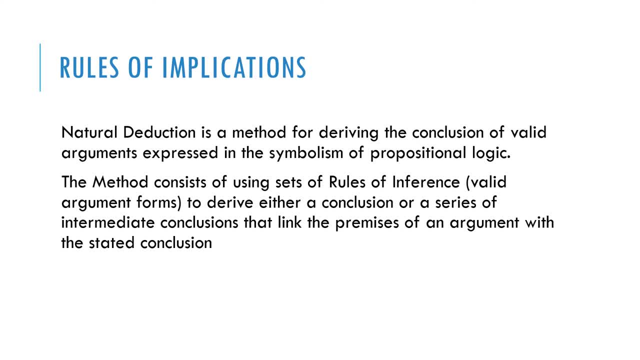 premises of an argument with the stated conclusion, we can use these rules to provide justification for what it is that we're trying to conclude, therefore being more confident in understanding what premises tell you and how we can justify a conclusion based on certain other premises. so, when you look back to 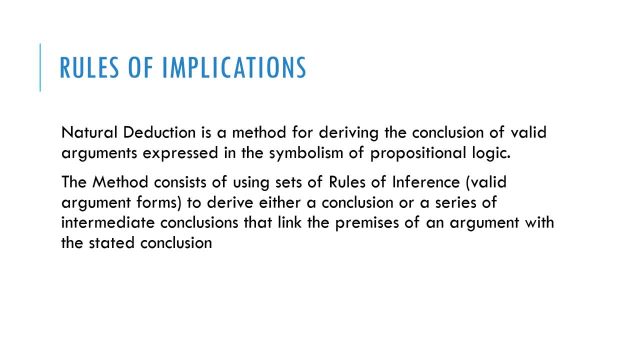 that word thought experiment that we opened up with. this is a very simplified and boiled-down version of natural deduction and doing a proof. now, you may not even know you were doing it, but essentially you were going through this method without necessarily knowing the correct rules of inference. but now, by learning, 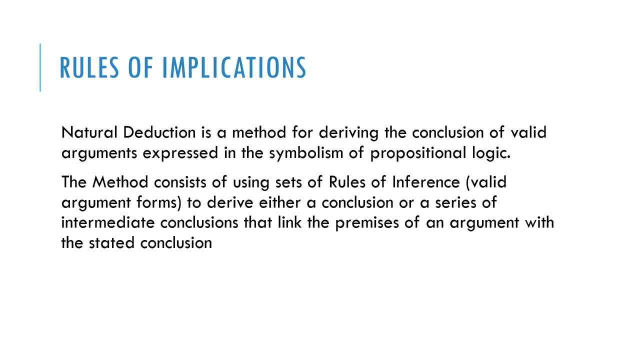 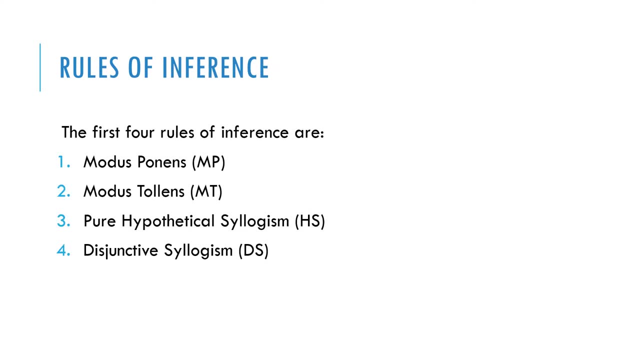 these rules, we can justify how we make the leap from premises to conclusion and know that the premises will support our conclusion and therefore justify what it is that we're trying to claim. the first four rules of inference are going to be modus ponens, modus tollens, hypothetical syllogism and 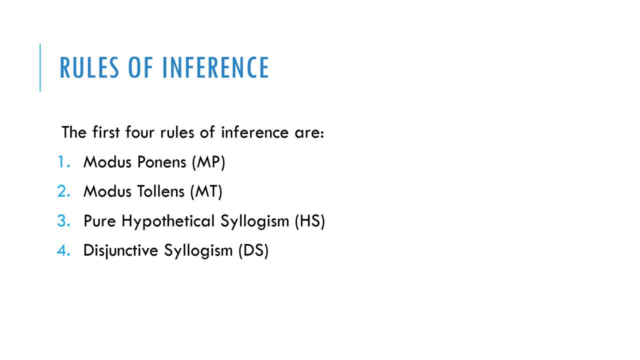 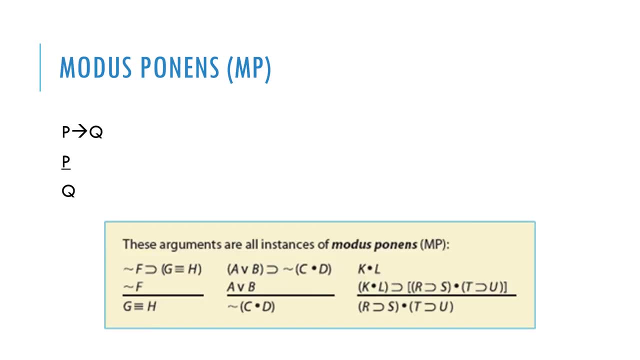 disjunctive syllogism. again, these are rules for how we can deduce certain information based on inference. take modus ponens, for instance. a modus ponens argument is one in which i use a conditional statement: if p, then q, and then affirm the antecedent p. 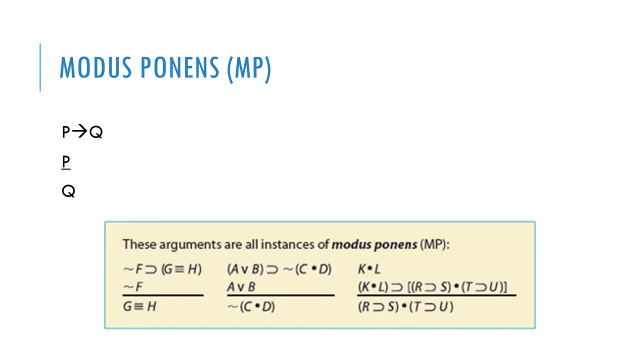 if i affirm the antecedent of a conditional, i am guaranteed to get my consequence. this means that i know that q is going to be true based on this argument form, because it follows this particular rule of inference known as modus ponens. in the box you can see other examples of much more complicated arguments that 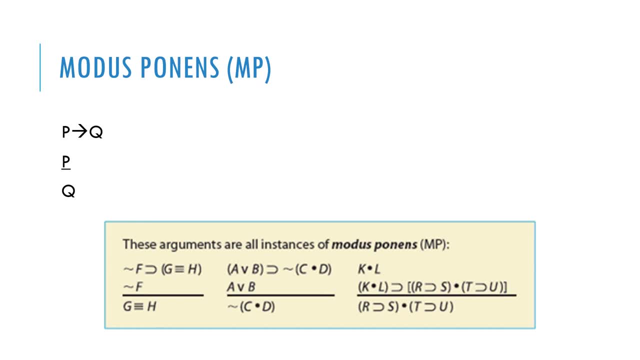 are expanded on of this boiled down version of: if p then q, p therefore q. so in the first argument, uh, in the box, we can see that if not f, then g, if and only if h, and then we affirm not f. so we must know that we get. 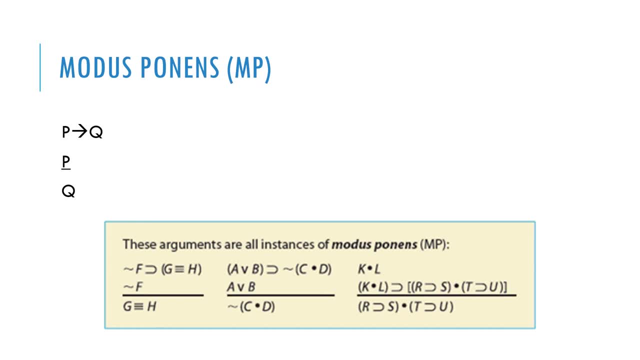 g, if, and only if h, because of the rule of inference known as modus ponens, and we can do that with the other two arguments in the box. so we know, with this particular argument form, we are always going to have valid arguments when we follow this. 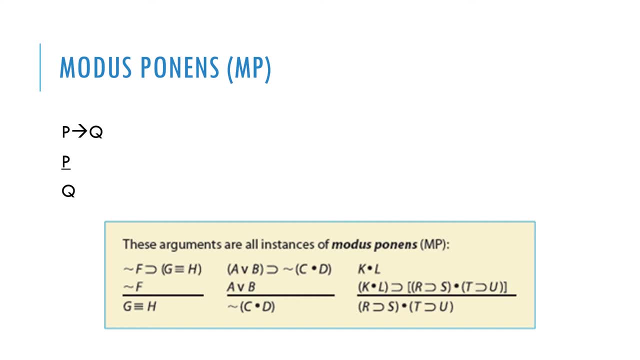 and we can justify why the argument is true, based on this particular rule of inference, modus ponens. the next rule is the modus tolens rule, and this has a very similar type structure to modus ponens in that it requires a conditional statement: if p, then q, but here let's call this case. 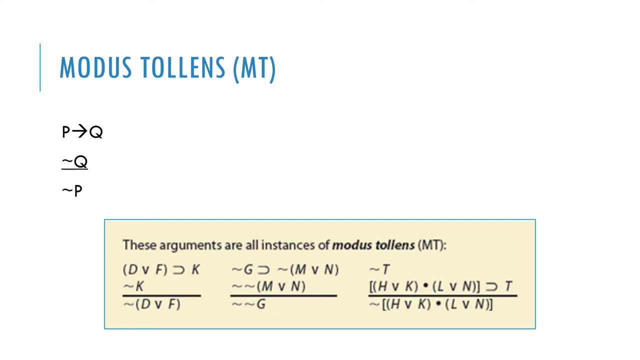 here we're negating Q and therefore, as a conclusion, we get not P. So if I suggest that P refers to holding a banana and Q refers to me holding something that's yellow, I can make the statement that if I'm holding a banana P, then I must be holding something yellow Q. But then I say: 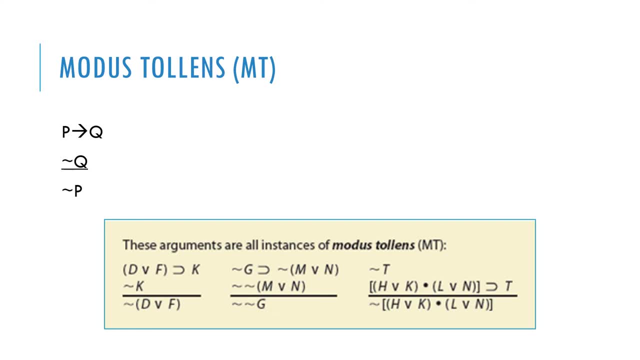 that I'm not holding something yellow, so we can therefore deduce that I'm not holding a banana. So here this rule is the modus tollens rule, in which we negate the consequent of a conditional statement and therefore get the negation of the antecedent. The arguments in the box are expanded. 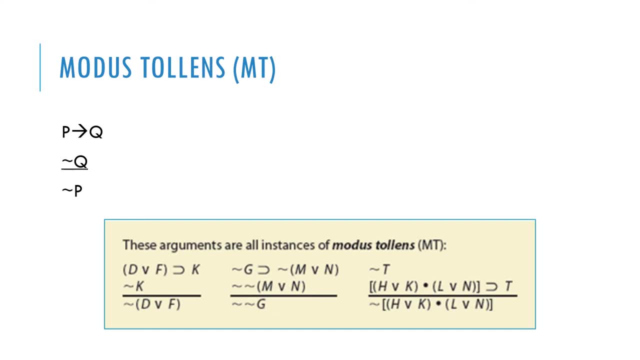 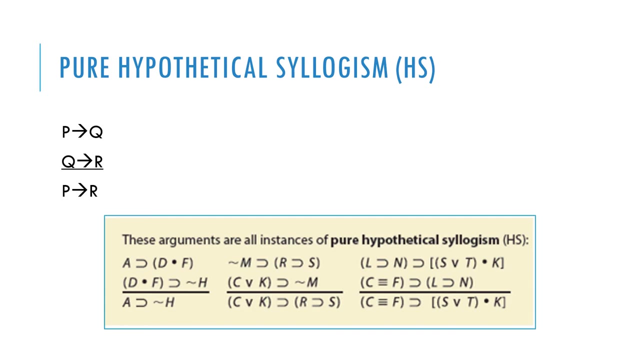 on in more complicated versions of the same argument structure. These are good argument structures that are not holding something yellow. So if I suggest that P is not holding something, that we can justify using the modus tollen rule of inference. The next rule is the hypothetical syllogism. The hypothetical syllogism states that if P is Q, 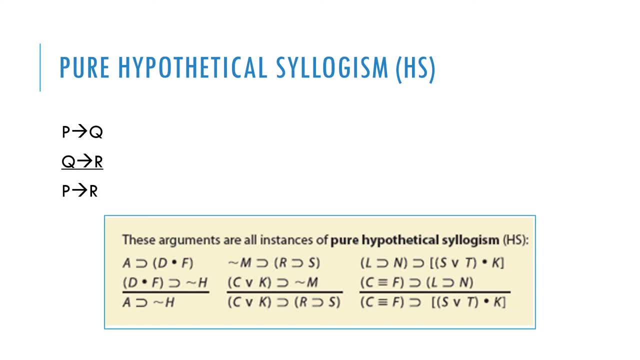 then Q must be true, and if Q is true, then R is true. With those two premises, I can therefore guarantee that if P is true, R must be true, And I do this through the argument structure of hypothetical syllogisms. We often refer to these as chain arguments because we can see that 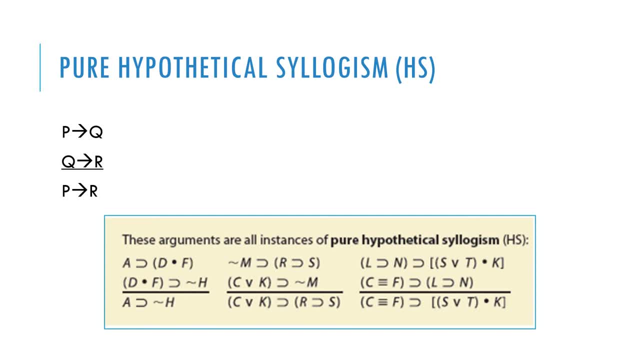 going in a chain: if P then Q, if Q then R. maybe if I were to say after that, if R then T, if T then S, then we can start from the first P that we mentioned and then lead it all the way down to S. And so these rules are important justification tools in order to 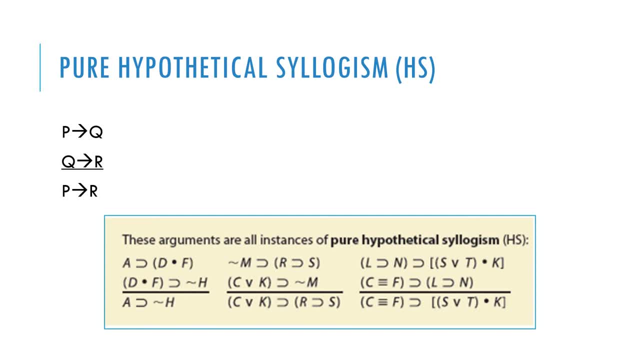 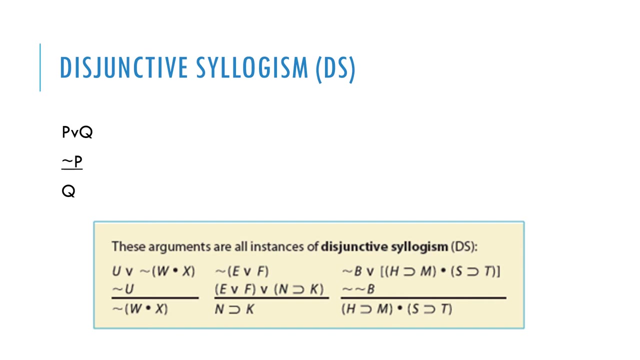 or determine whether or not arguments are valid and to deduce naturally intermediary conclusions. the next is the disjunctive syllogism. the disjunctive syllogism states that P or Q, and then if not P is true, then Q must be true. so here you can see where 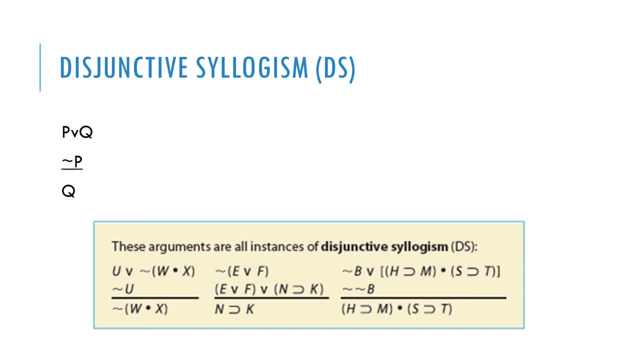 we're using in either or statement saying that either P is true or Q is true. if I know that P is not true, then it must be the case that Q is true again. these rules will help us to recognize whether arguments are valid and will help us inform, help us form valid arguments and then justify those. 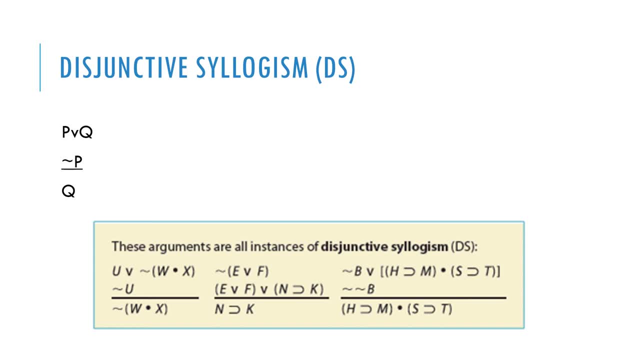 arguments that we or others make, so that we know whether or not particular arguments are going to be valid or invalid. after we understand these proofs, we can always, therefore, put arguments into truth tables to know for certain whether or not an argument is going to be valid or invalid. this will essentially save time. 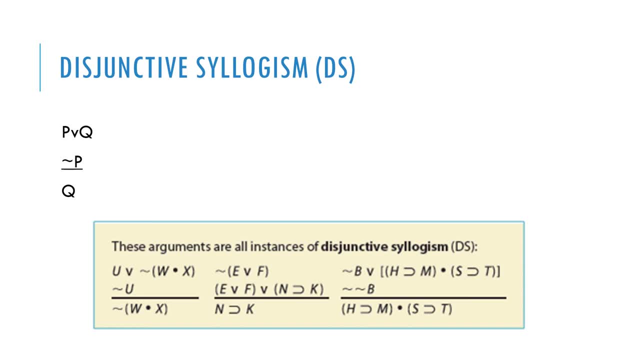 by learning different argument forms, so we're not always having to use truth tables in order to determine whether or not an argument is going to be valid or invalid. we can simply just memorize these rules and then recognize those forms when you see them. so this will help in terms of finding out. 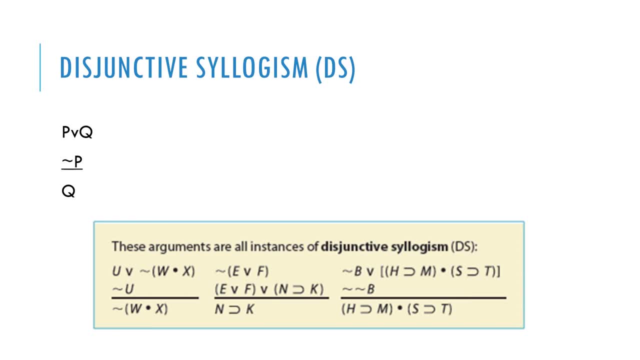 whether or not, or determining whether or not an argument is valid or invalid, prior to even creating a truth table. we're able to memorize these rules and then, when we see an argument, see if it backs up, follows one of these rules or if we can use multiple rules, as in the complicated argument. 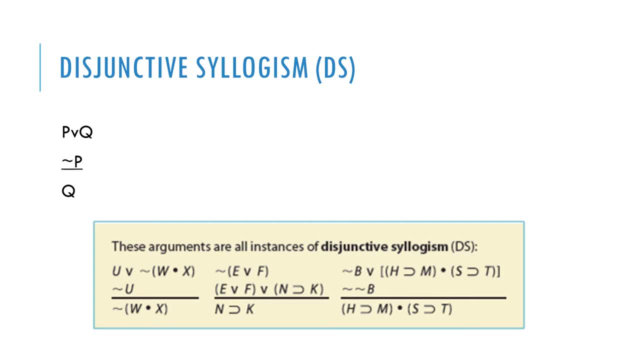 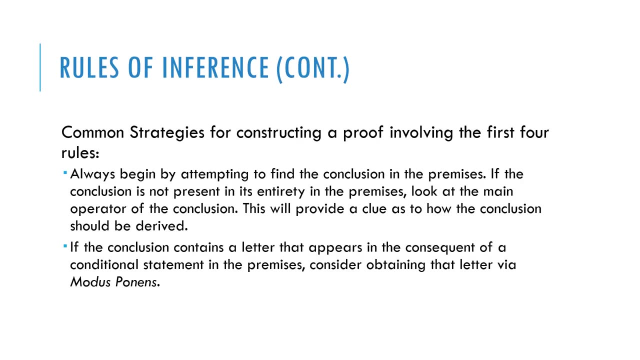 shown previously and therefore deduce some conclusion from it. Now, when it comes to these rules of inference, there are common strategies for constructing the proof. For instance, we can always begin by attempting to find the conclusion in the premises. If that conclusion is not present, then the premises look at the main operator. 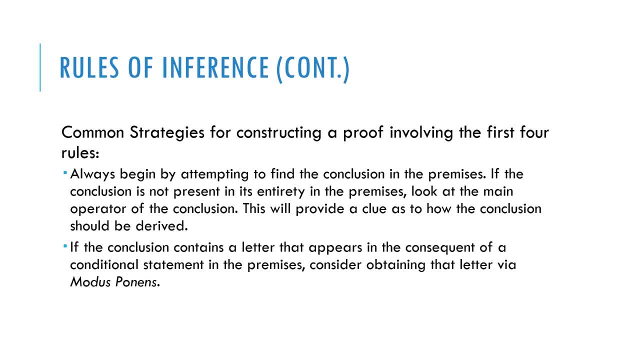 of the conclusion. This will provide a clue as to how the conclusion should be derived. If the conclusion contains a letter that appears in the consequent of a conditional statement in the premises, then consider obtaining that letter via modus ponens. So again, 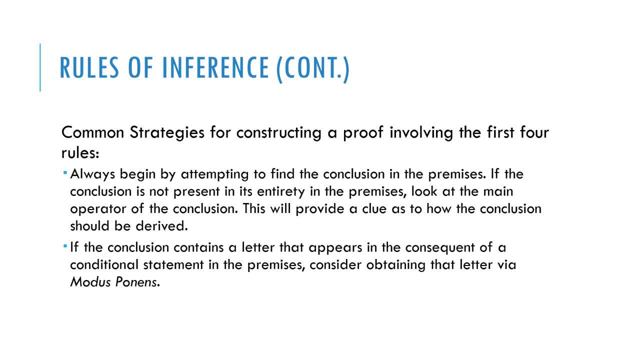 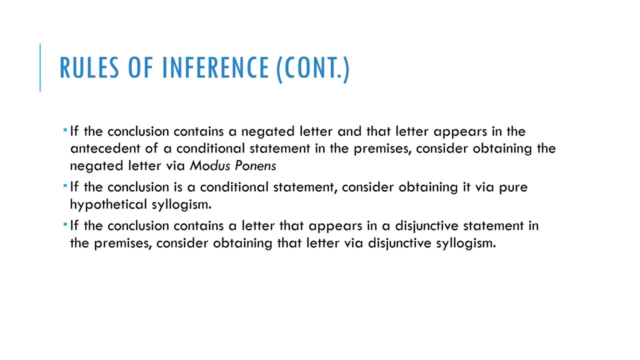 we can use modus ponens arguments or modus tollens arguments, depending on how an argument is structured, in order to derive a conclusion or justify why a conclusion is the way that it is. Also, we might think that if a conclusion contains a negated letter, that that letter 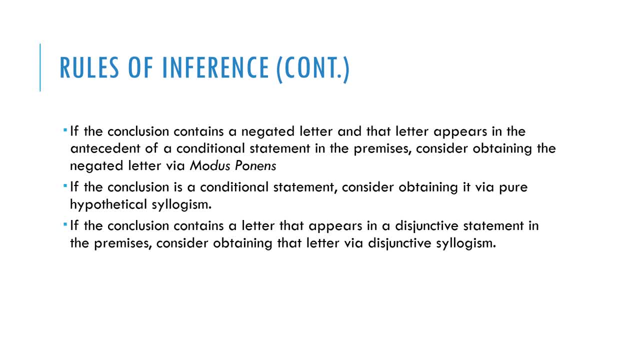 appears in the antecedent of a conditional statement in the premises, then we might obtain that negation. If the conclusion contains a negated letter via modus ponens arguments or modus tollens arguments, then we might obtain that negated letter via modus ponens arguments or modus. 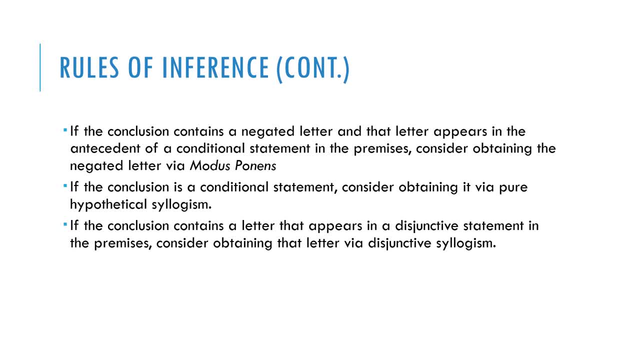 tollens arguments or modus tollens arguments. So remember, modus ponens is the argument structure. if P, then Q, then I affirm P. therefore I must get Q. If, on the other hand, a conclusion is a conditional statement, consider obtaining it via pure. 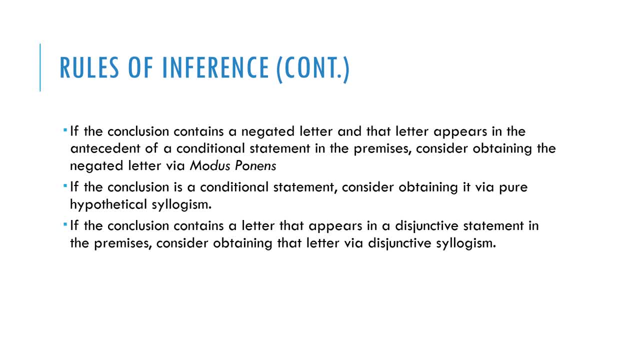 hypothetical syllogism. So again, we can get to a conclusion through chain argument using a hypothetical syllogism: If P then Q, if Q then R. we must therefore know that if P, then R. Next, if the conclusion contains a letter that appears in a disjunctive statement, then 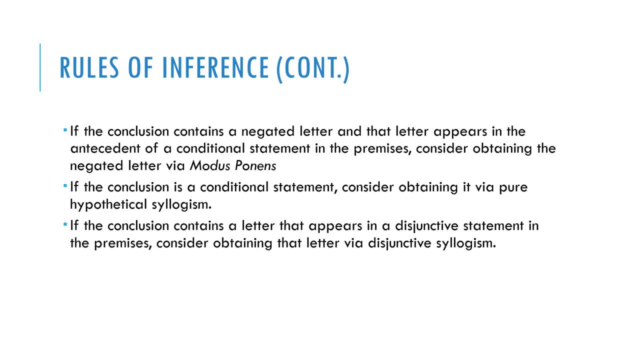 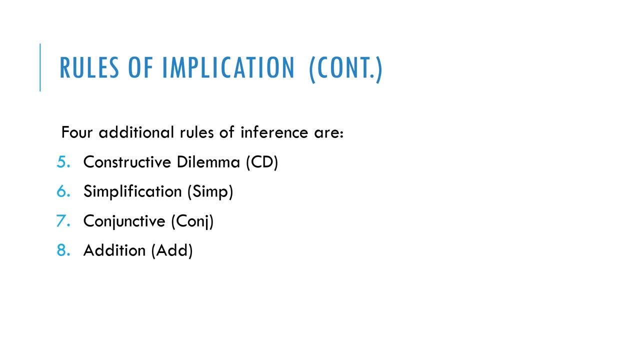 consider obtaining that letter via disjunctive syllogism, So P or R, and then we suggest that not P is true. we must therefore know that Q is true. Now, in addition to rules of inference, there are also rules of implication. 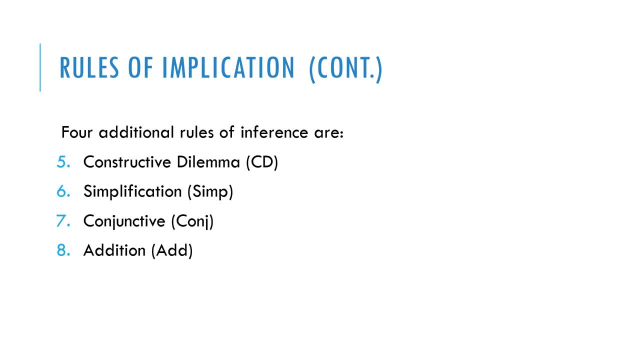 And all of these rules should be memorized to the best of your ability because, again, they will help us justify valid arguments, they will justify conclusions based on how premises are laid out. So, in addition to the rules of inference, there are four rules of inference that we 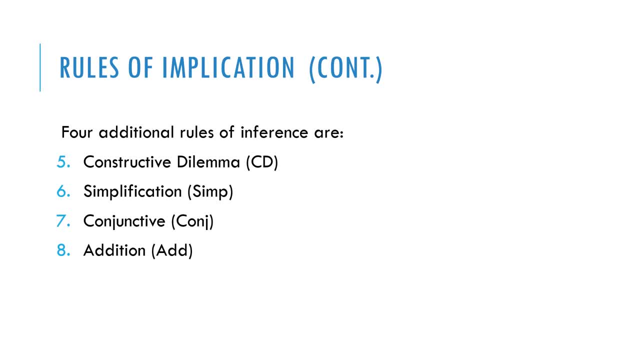 can use to solve the problem. These rules of implication also are rules of inference, just a subcategory of the rules of inference, and they are the Constructive, Dilemma, Simplification, Conjunctive and Addition. Notice how each of these rules of inference has a subcategory. 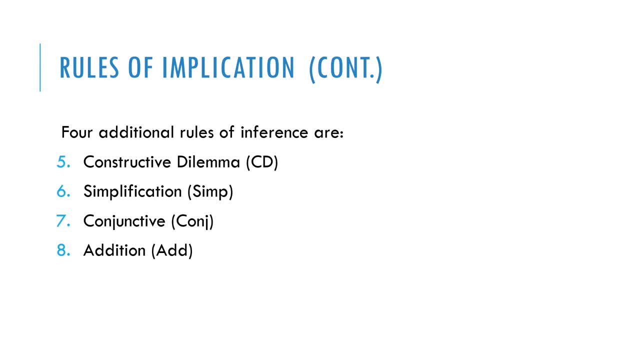 So in this case we have the Constructive Dilemma: Simplification, Conjunctive and Addition. Notice how each of these rules of inference are. subcategory of inference has a acronym or abbreviation that allows us to shorthand justify which rule we're using at any given time. Now the constructive dilemma. 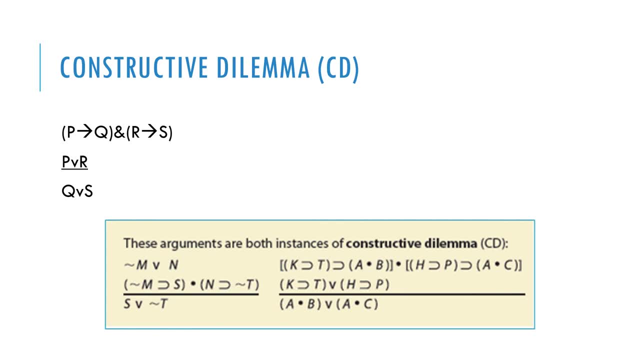 is going to be the first additional rule we look at, and so here we can see: if we have an argument, if P, then Q, and if R then F, and we know that P or R is true, then we can therefore deduce that Q or F has to be true. So again, we go through. 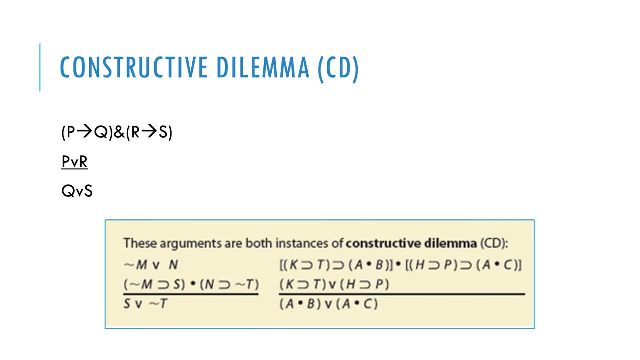 and try to memorize or familiarize ourselves with the rules in order to help justify certain steps we make in the natural deductive process, so that if we're questioned on how we can get to a certain conclusion, we can say that well, based on the constructive dilemma and based on modus. 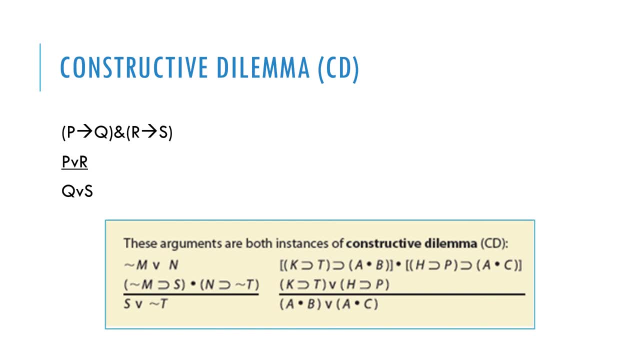 ponens, we can see these lines and these lines, and therefore it must be true that this conclusion is the case, And so knowing these rules will help us familiarize ourselves and and be more confident in the way that we justify ourselves and more confident in understanding word problems or problems. 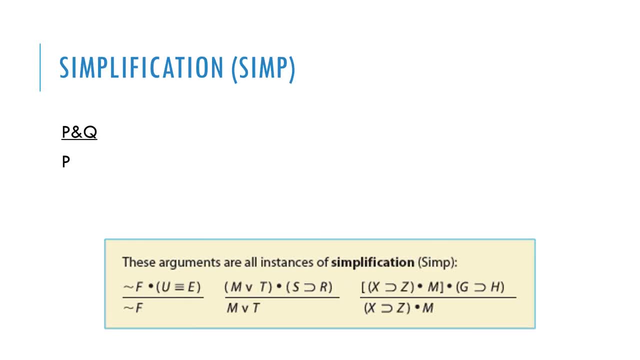 that may arrive that require natural deduction. The next rule is simplification, and this is a pretty easy rule. if I were to say that P and Q is true, then I would know that P is true. I would also know that Q is true because, remember, when I use a conjunctive claim- P and Q- it must be the case that both. 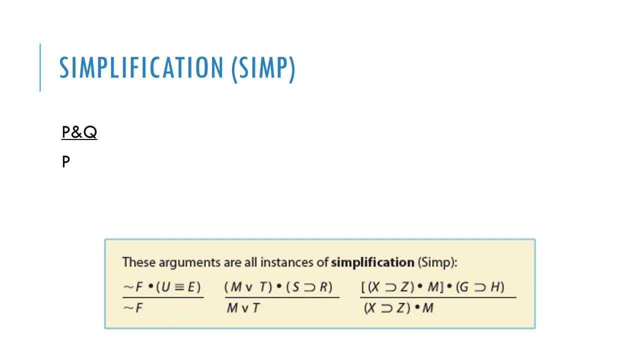 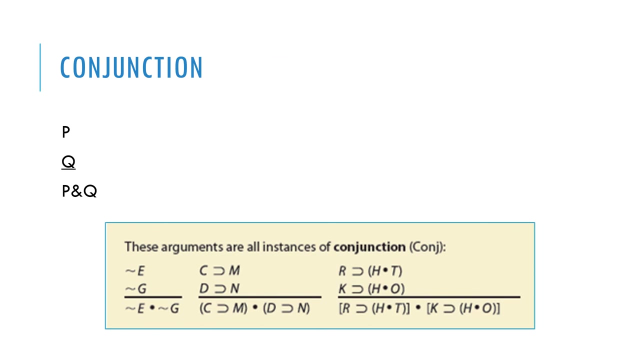 are true. Down in the box, you will see more complicated examples of this, as they may appear in real life. Next is the conjunction, and the conjunction is a fairly simple one as well, one that we've already talked about: this idea that if I know that P is true and I know that Q is true, then it must be the case that 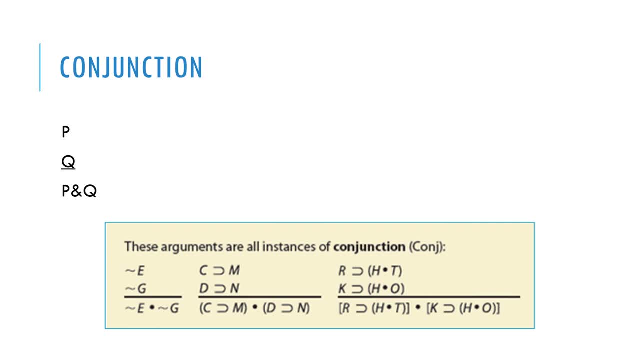 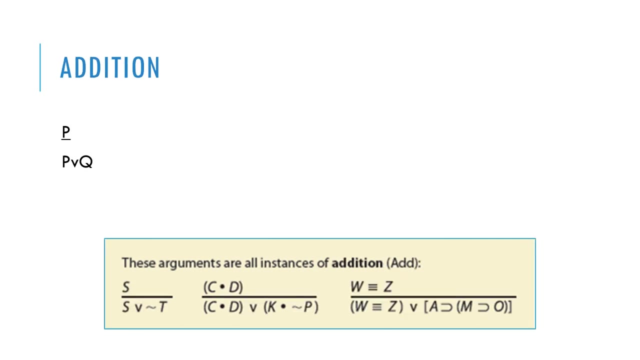 P and Q is true. Again, here we're just combining premises using a conjunctive and and therefore I know that the complex proposition is true when each of the simple propositions is true. Lastly, is the rule of addition and so that, if I know that P is true, I can therefore add anything to. 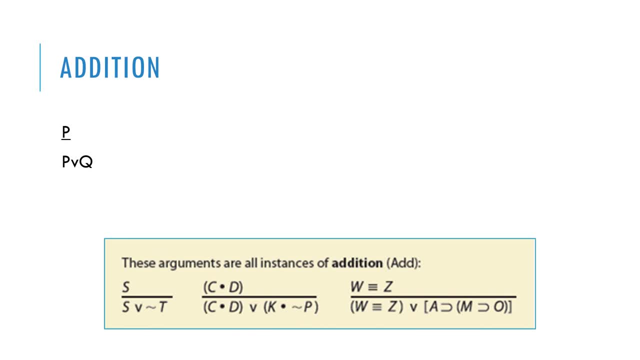 P with the disjunctive or. So if I know that P is true, then I can make the claim that P or Q is true, or I can make the claim that P or S is true or P or anything else. If I know that one side of a disjunction is true, or if I know that 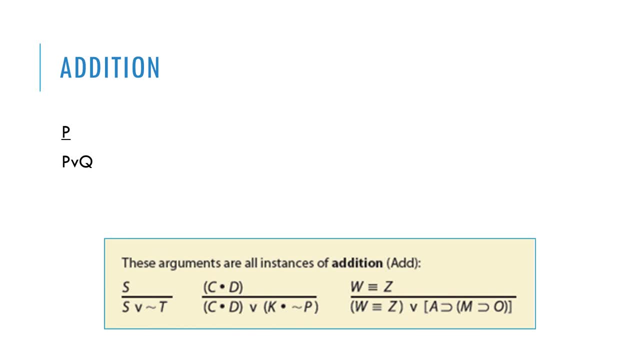 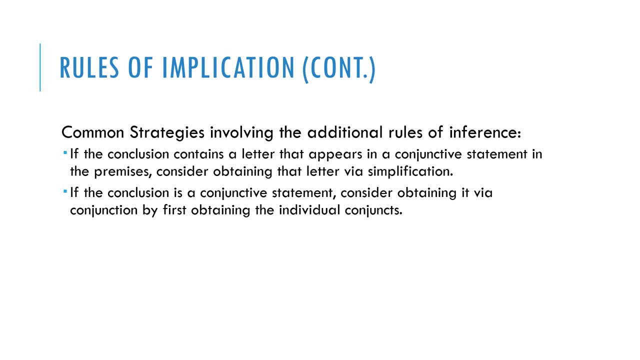 something is true, I can add any kind of disjunctive claim to it, and it still remains true. So now, with these rules of implication, certain strategies, we can look for that if a conclusion contains a letter that appears in a conjunctive statement. so a 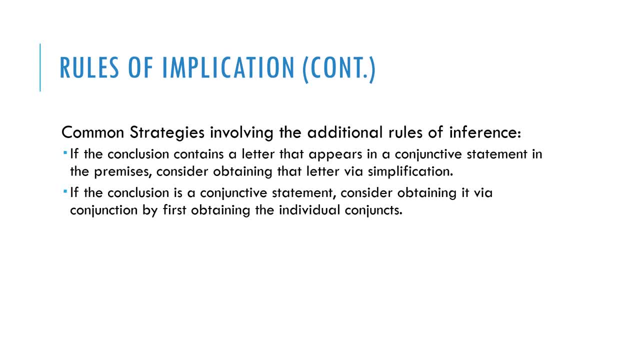 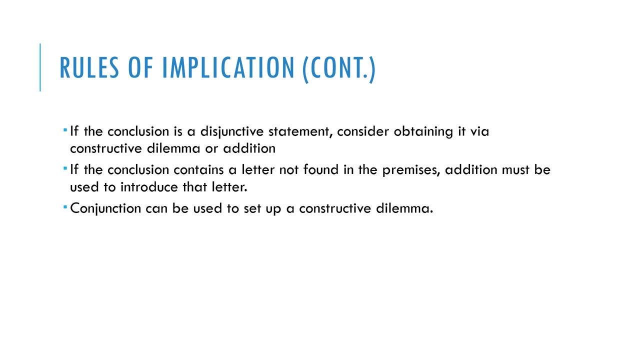 and statement within the premises, consider obtaining that letter via simplification and if the conclusion is a conjunctive statement, consider obtaining it by a conjunction, by first obtaining the individual conjunct. Also, when we look and see that if the conclusion is a disjunctive statement, 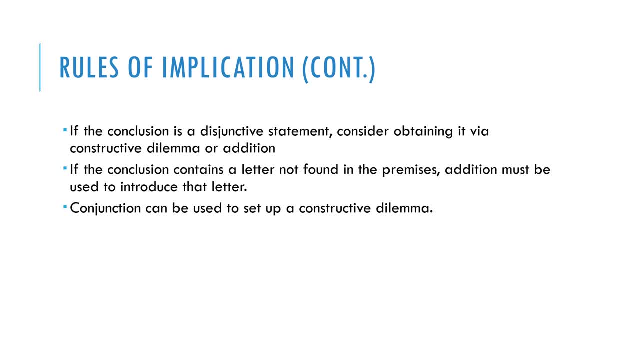 consider obtaining it by a constructive dilemma or addition. If the conclusion contains a letter not found in the premises, then addition must be used to introduce a new letter, just like we did that if we know that P is true, then we can say P or Q, or P or S, and then, lastly, conjunctions can be used to set up a. constructive dilemma. Thank you very much.